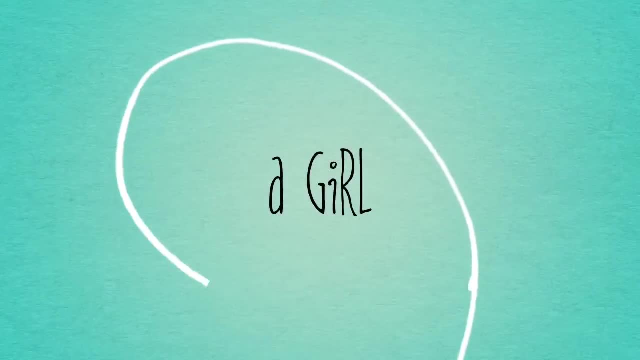 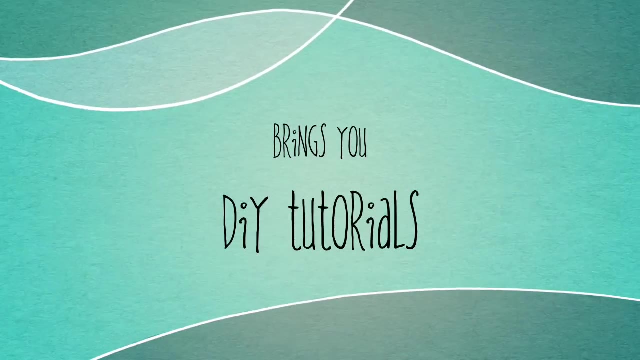 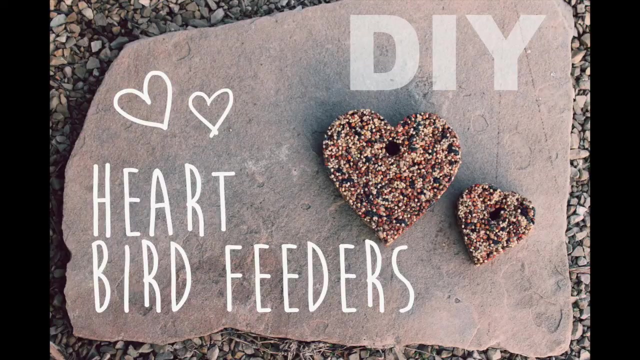 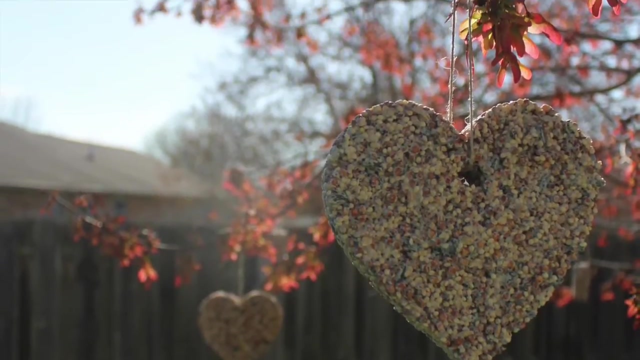 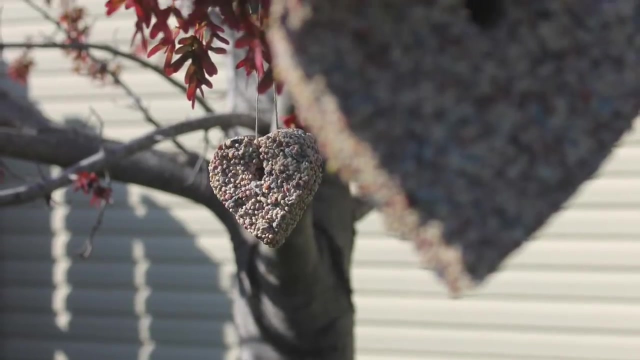 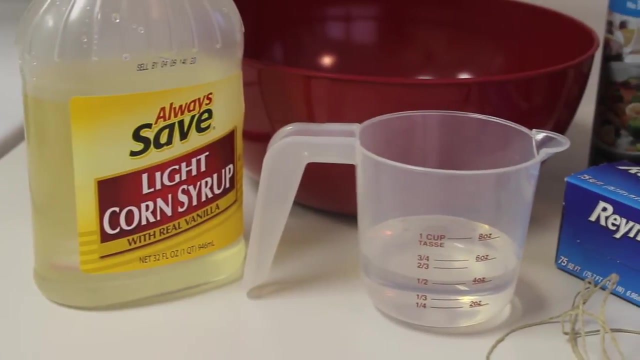 Hey guys, today I want to share with you a really cute craft that is super easy to make, eco-friendly and inexpensive. These heart-shaped bird feeders make a perfect addition outside of your home and attract beautiful birds during the springtime. To create these bird feeders you will need corn syrup, a large mixing bowl, water, non-stick. 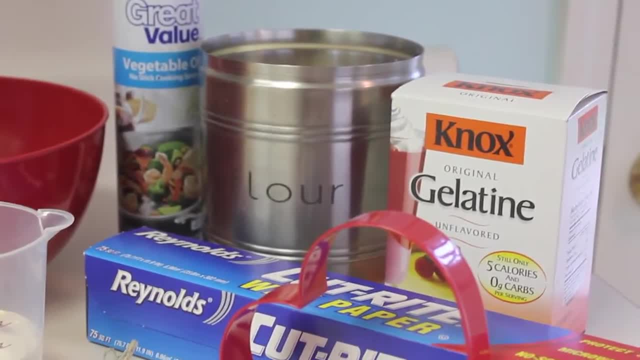 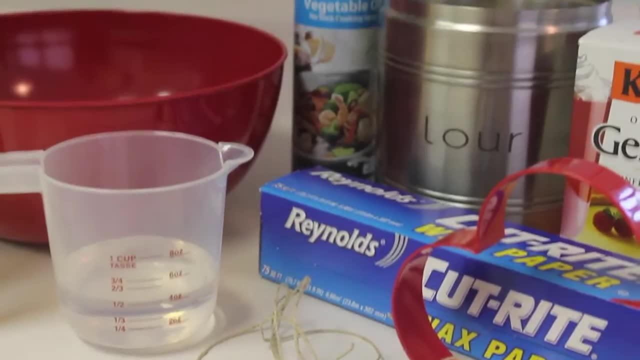 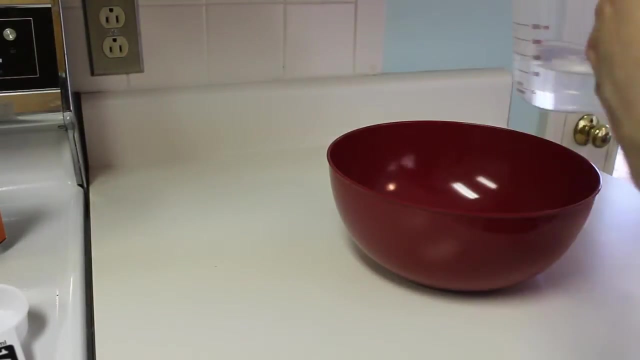 spray, wax, paper, flour, a heart-shaped cookie cutter, gelatin and twine, And not pictured here. you will also need a straw or a marker lid, something you will be able to make a hole for your bird feeder and, of course, bird seed. To get started, you're going to 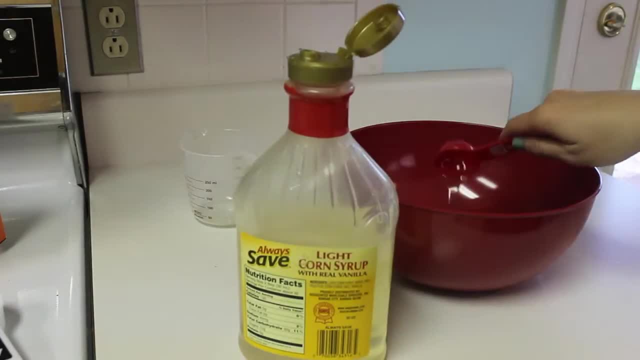 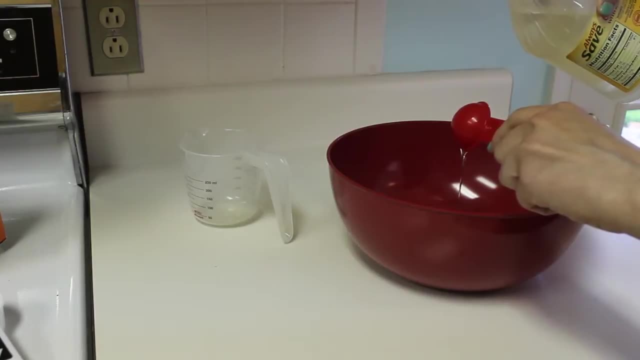 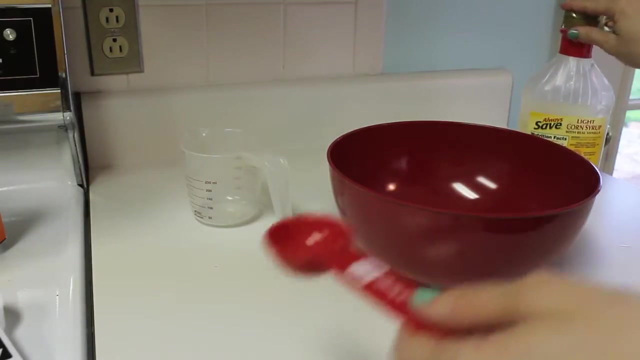 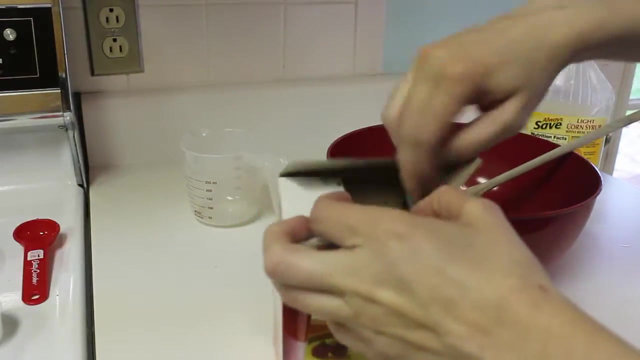 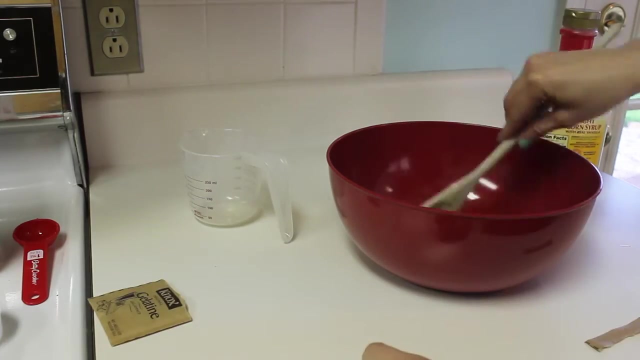 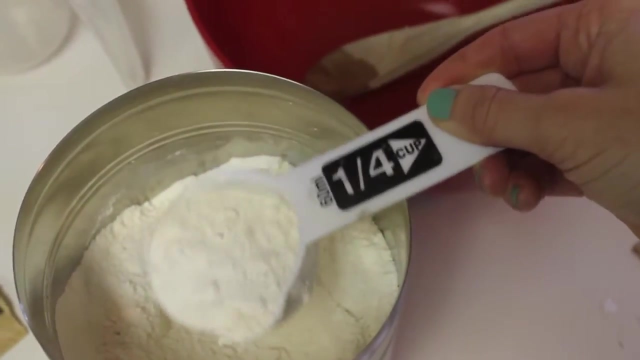 be adding 1 1⁄2 cup water and 3 tablespoons of corn syrup to your mixing bowl. Now I'm going to be adding 1 envelope of unflavored gelatin to the mixture. Once you have stirred your water, gelatin and corn syrup together, add 3⁄4 cup flour to the 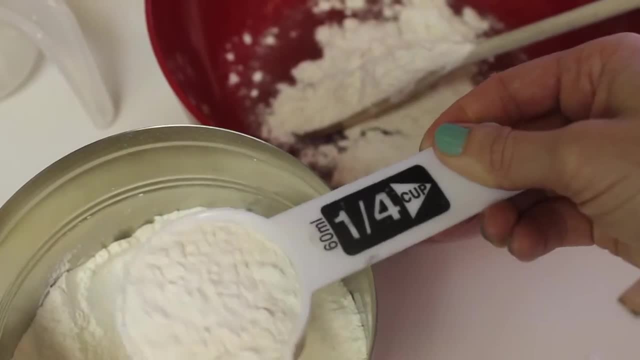 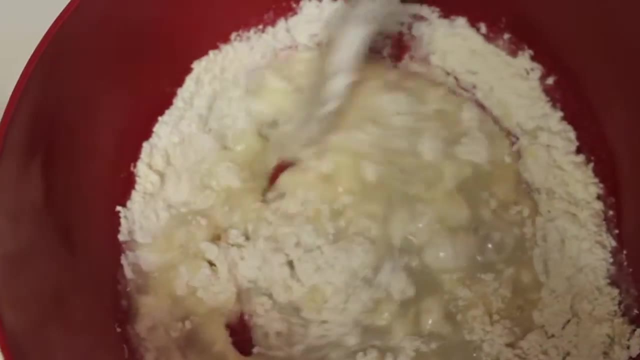 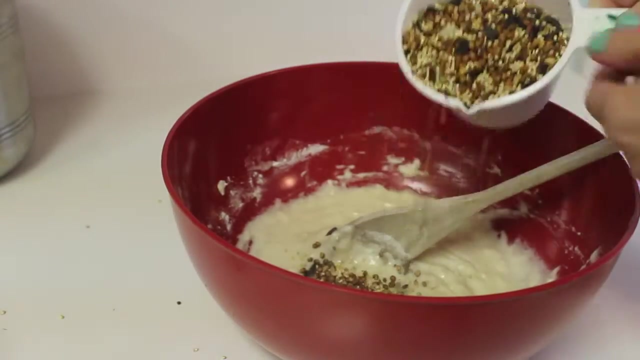 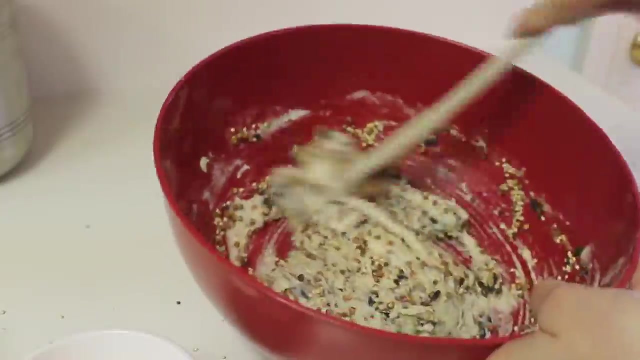 bowl. Mix all of your ingredients thoroughly into a batter. It should look something like pancake batter when it's all mixed together. Our last step is to add our bird seed. I'm going to be adding 4 cups of bird seed to the mixture and stirring it as I go. 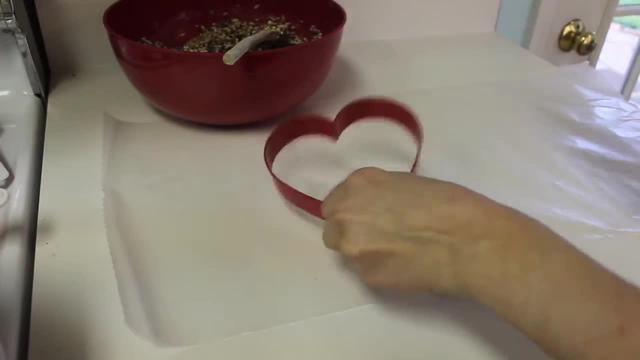 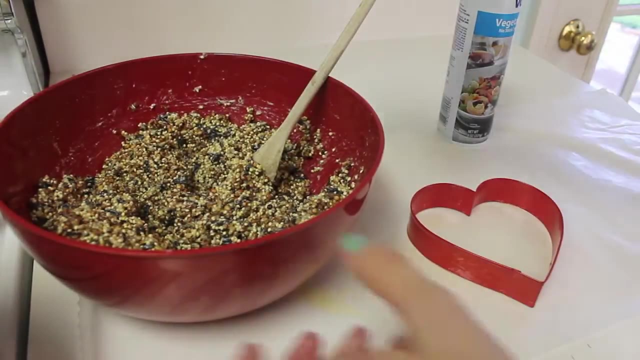 When your bird seed mixture is thoroughly combined, you're going to want to add a little bit of sugar. You can also add a little bit of salt. Use some non-stick spray on the inside of your cookie cutter to prevent the bird seed from sticking.